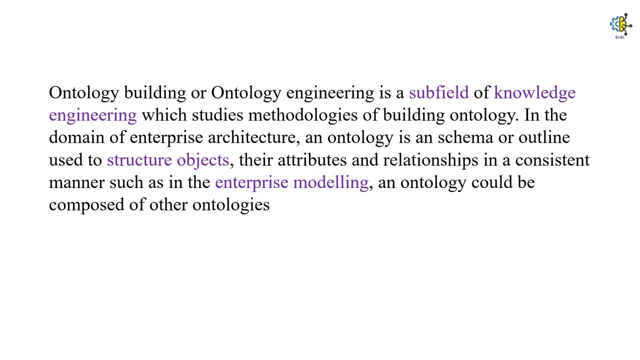 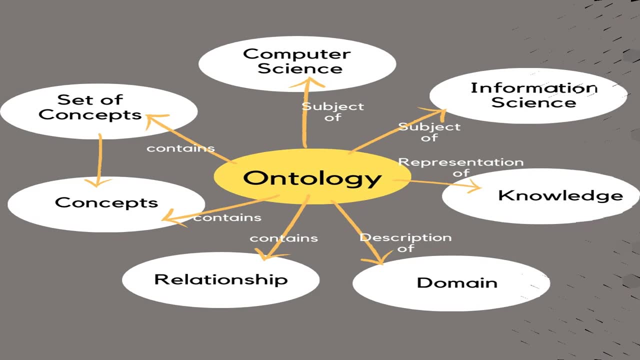 But these different, similar and dissimilar ontologies can also be connected together to form a bigger image, bigger perspective. In this image on your screen you can see ontological significance. So ontological is a subject of computer science and information science, as I said earlier. 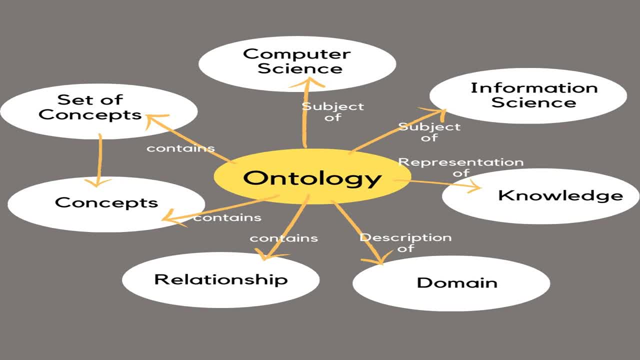 What does ontology represents? Ontology represents knowledge. What does this ontology describes? This ontology is description of domains, various domains, various interconnected domains, and interconnected domains too, And, finally, what this ontology contains in itself. So, as I told you earlier, ontology contains relationships, concepts. 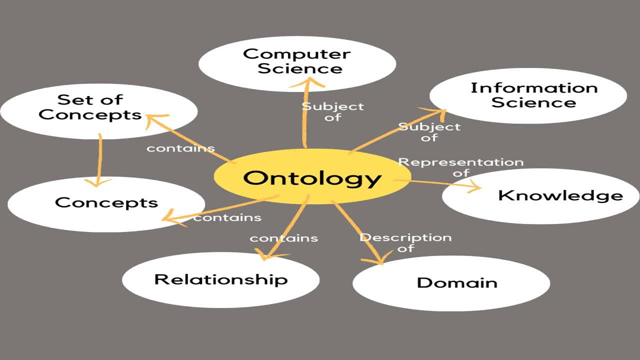 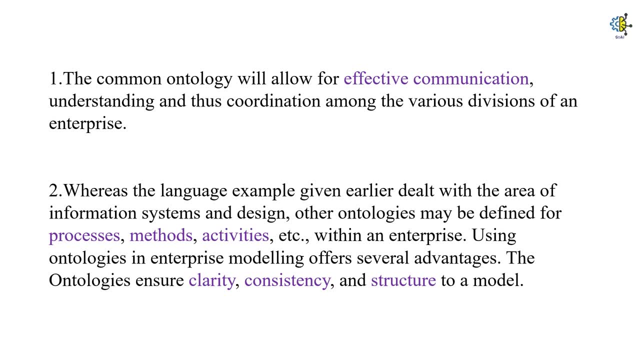 and different sets of concepts all together. So this is our ontology. Now, the common ontology will allow for effective communication Where In the different objects among the different objects, And it will help different objects in an enterprise to coordinate among each other. 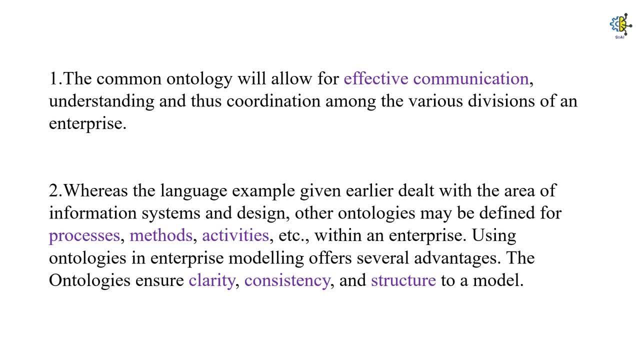 Be it the same division or the other division. Here is a language example which deals with information science only and designing only, But there are various other ontologies which are defined in the process making, method, structuring and activities planning. also. All these ontologies and processes will be within an enterprise. 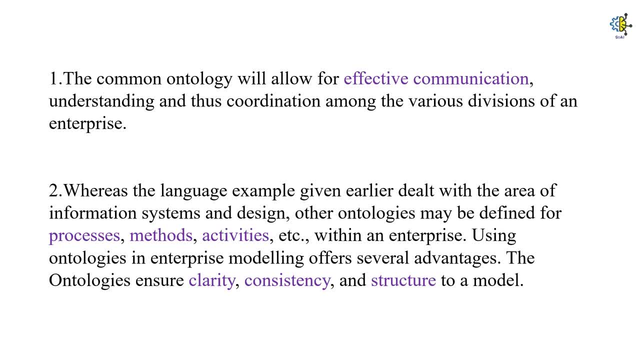 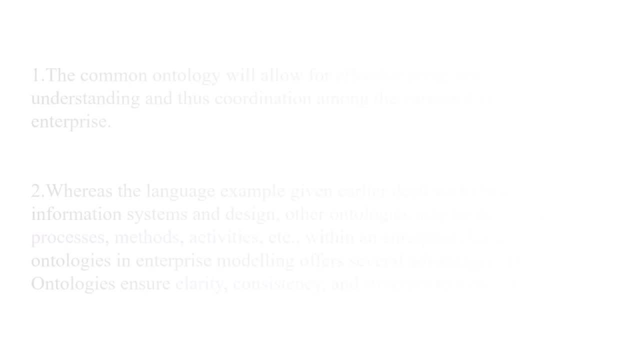 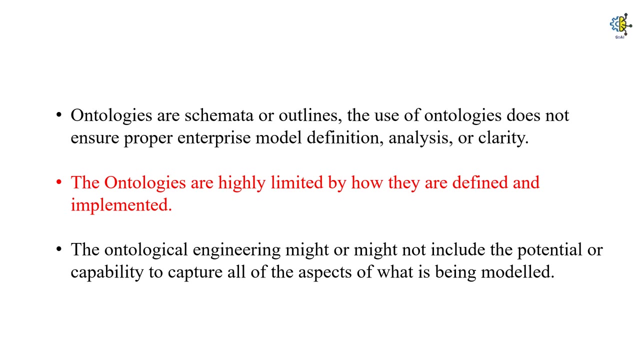 These ontologies in the enterprise modeling not only offer several advantages, but also it shows the clarity, consistency and structure of a model. What do we mean by enterprise? I will tell you shortly with an example. So ontologies, as I said, are schemas, or outlining, or structuring architecture of the objects and their relationships. 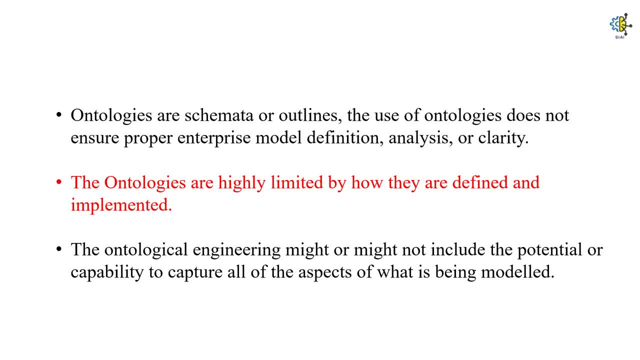 But one thing I want to make sure: that simply the use of ontologies does not ensure the proper enterprise model definition. It does not mean that, okay, we have defined the ontologies and our work is done. No, In an enterprise model definition, analysis and clarity not only comes from ontologies but from various other aspects also. 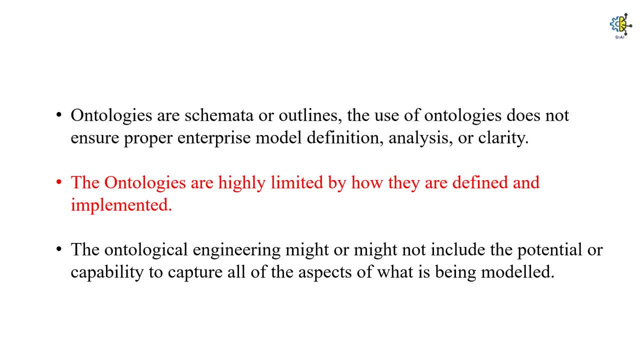 Ontologies can be, at times, very limited in the manner in which they were defined, So their definition limits their abilities and potential, and vice versa. Also, the ontological engineering might or might not include the potential or capability to capture all of the aspects of what is being modelled. 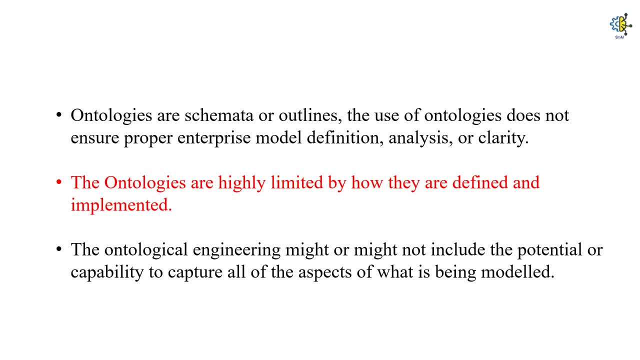 What does this mean? It means that ontological engineering may be or may be not be possible to capture all aspects of the enterprise model. Potential and capabilities should be included, All aspects of the enterprise model. We have already discussed this in the previous example. 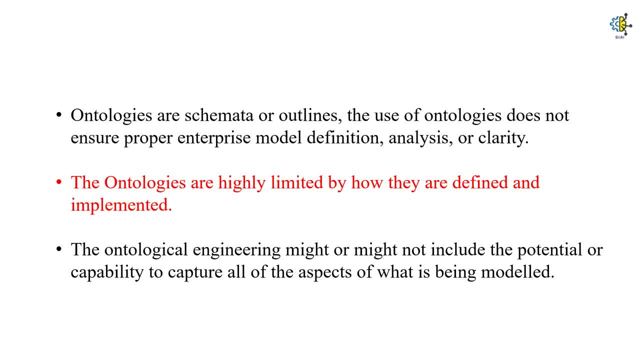 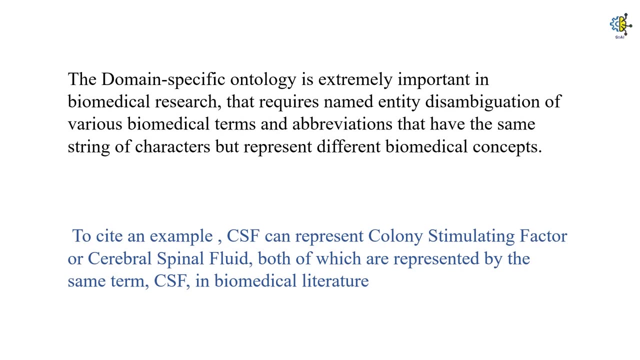 The modelling of ontologies is limited in their definition and implementation methods. There are various domain specific ontologies. also, One such domain specific ontology is highly sought in biomedical research. Why? Because biomedical research is highly sought. Why? Because biomedical research is highly sought. 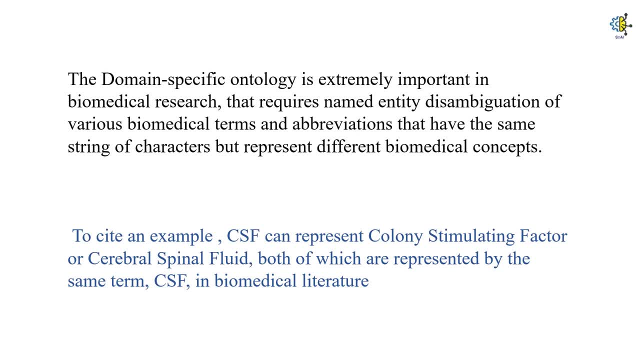 Because it requires various named entity. For example, CSF can represent colony stimulating factor. For example, CSF can represent colony stimulating factor. at the very same time it can represent cerebral spinal fluid. so we can see, here only CSF can be used to represent both of the terms, but they both have a different diaspora, different. 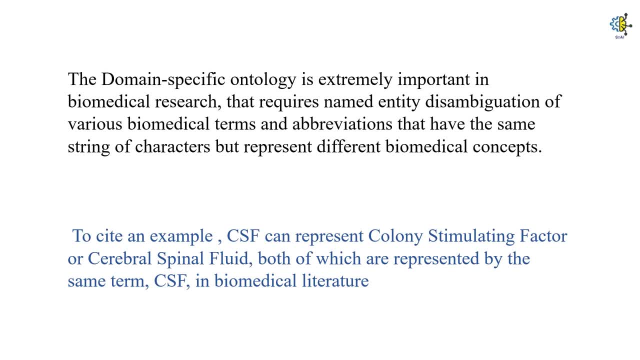 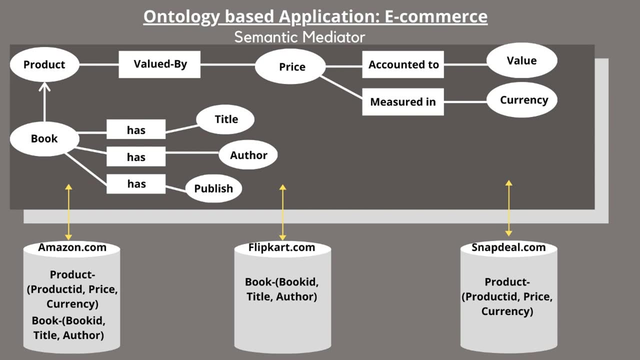 meaning and different application field, and they both are regulated, connected, in the biomedical literature. only now I will give you an example of what enterprise refers to. so an enterprise, basically this collection of various objects, outsourcing of those objects and consentencing of those objects. for example, if an enterprise sells the product, then the method by which those 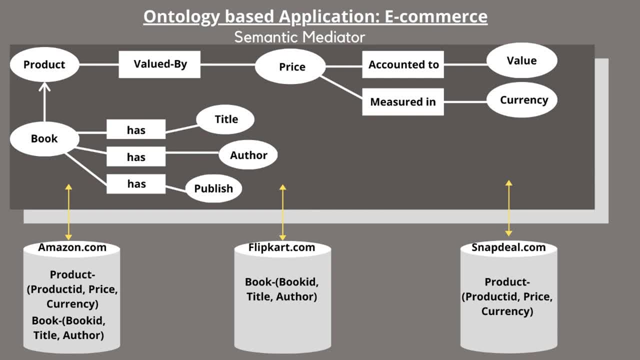 product will be valued will be their price, and this price will be further either accounted or will be measured. when we will account the price of a product, we will be working on the value of the product, the market value, the market capitalization of that product. but when we will measure the, 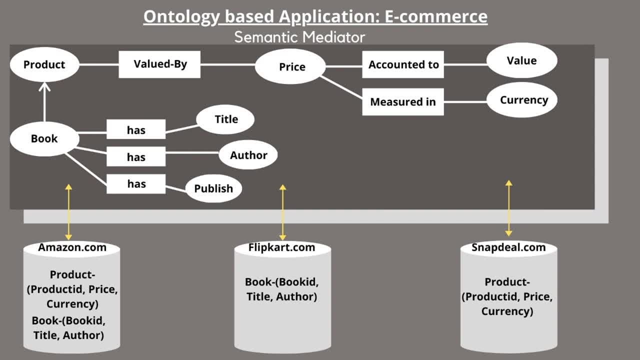 price of the product. we will be working in currency of that price and not with market capitalization. A book will be having a title for sure, an order for sure and a publisher for sure. The various examples of these enterprise products are specific for each one of these products. you can see here- and this was the example of enterprise- The book is the product and we are not talking about the price, we are talking about its contents, Its abilities and potential. then the book, if a product is a book, then book will have a title for sure and order for sure and a publisher for sure. 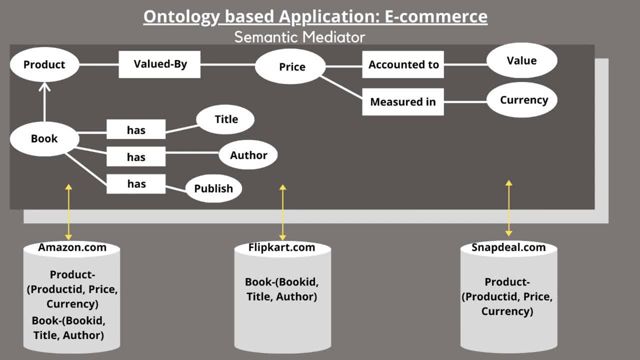 if we talk about e-commerce industries, it will be Amazon, flipkart, snapdeal. their product will have product ID. they will have price. price will be measured in value and currency. also this, this product, particularly book. if the product is book, then consecutively the book will have book ID, title and author. also this will 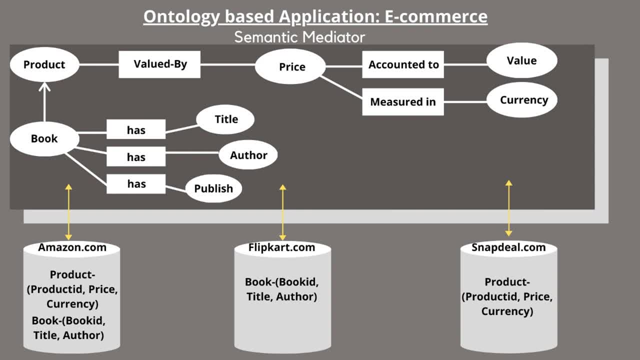 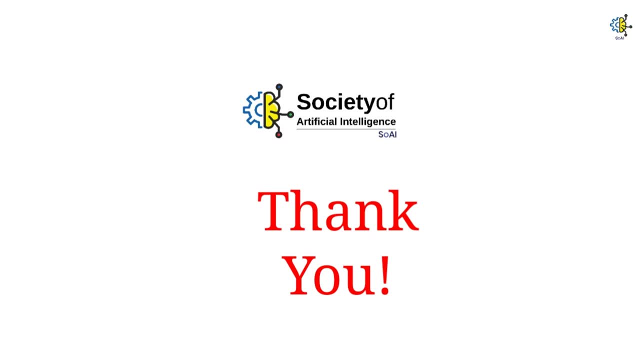 be same for various other enterprises in different domains also. with this, I hope you must have received a simpler gist of what ontological engineering is. thank you, have a nice day.